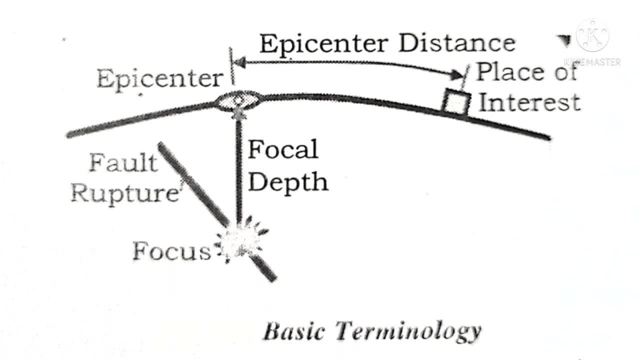 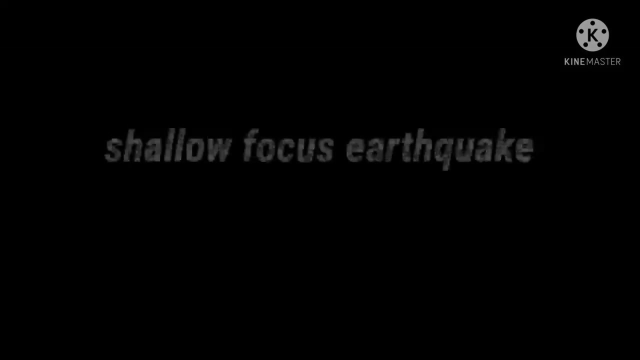 Focus or Hypo center. In earthquake, the waves emanate from a finite area of rocks. However, the point from which the waves first emanate or where the fault movement starts, is called the earthquake focus or hypo center, Epicenter. The point on the ground surface just above the focus is called the epicenter. 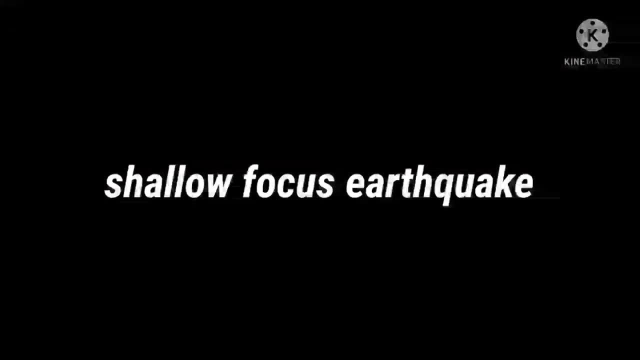 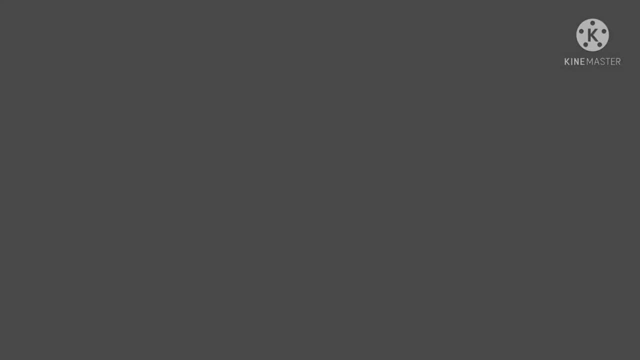 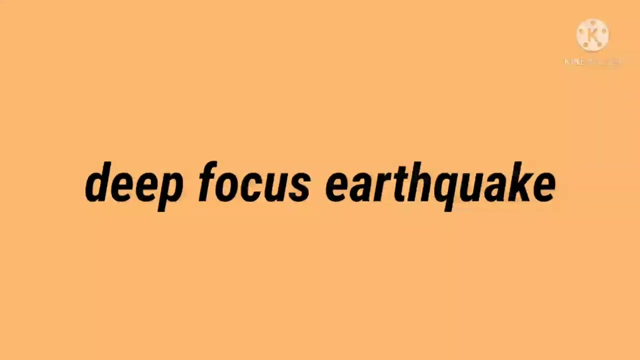 Shallow focus earthquake. Shallow focus earthquake occurs where the focus is less than 70 km deep from ground surface. Intermediate focus earthquake. Intermediate focus earthquake occurs where the focus is 70 km to 300 km deep from ground surface. Deep focus earthquake. Deep focus earthquake occurs where the depth 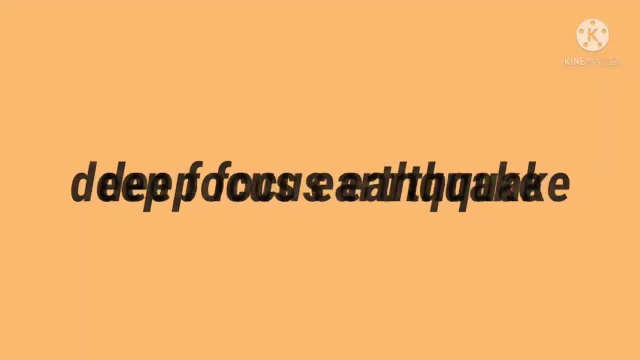 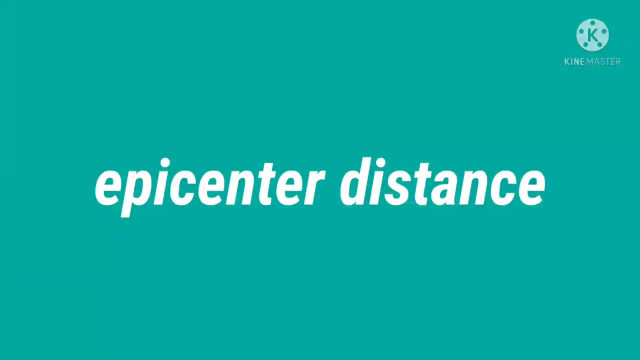 of focus is more than 300 km. Also non-det개를 focus long distance is called the epicenter distance. Discovery of very advanced theories is also one of rules. Distance between epicenter and recording station is kilometers, or in degrees is called epicenter. 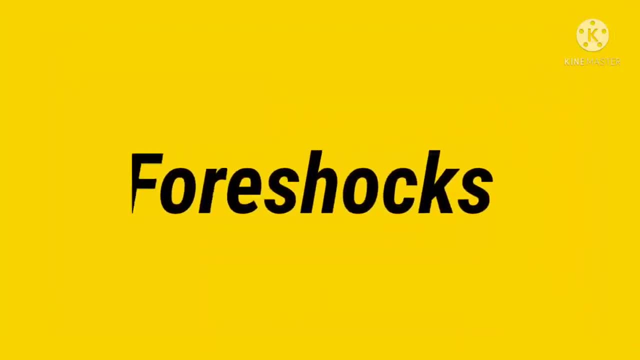 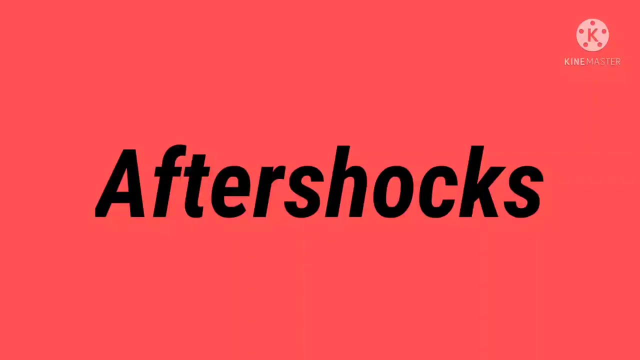 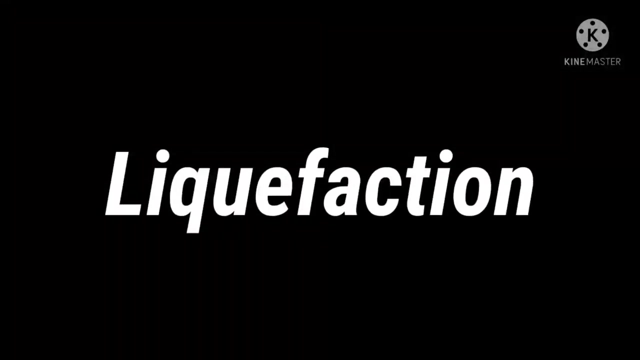 distance. Next is foreshocks. Foreshocks are similar earthquakes that precede the main earthquake. Next is aftershocks. Aftershocks are similar earthquakes that follow the main earthquake. Next is liquefaction. Liquefaction is a state in saturated, cohesionless soil wherein the effective shear strength 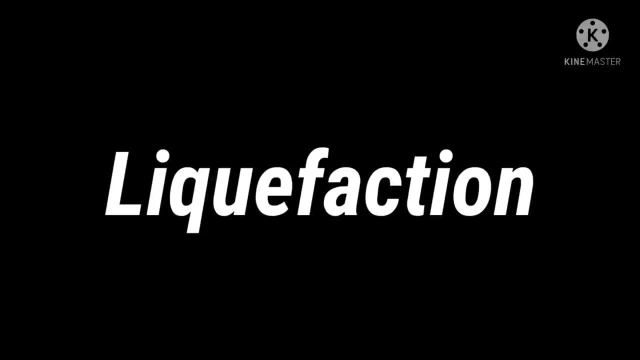 is reduced to negligible value for all engineering purposes due to pore pressure caused by vibration during an earthquake, when they approach the total confining pressure Leading to localס falqi e connection of earthquakes between temperatures. In this condition, the soil tends to behave like a fluid mass. 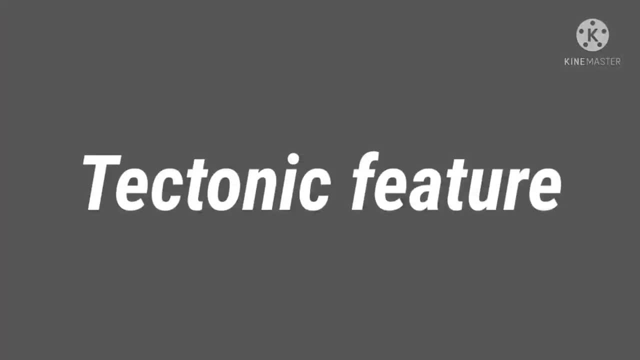 Tectonic feature, The nature of geological formation of the bedrock in the ground, revealing regions characterized by structural features such as dislocation, distortion faults, folding thrustThere wanna, volcanoes with their age of formation, which are directly involved in the earth. 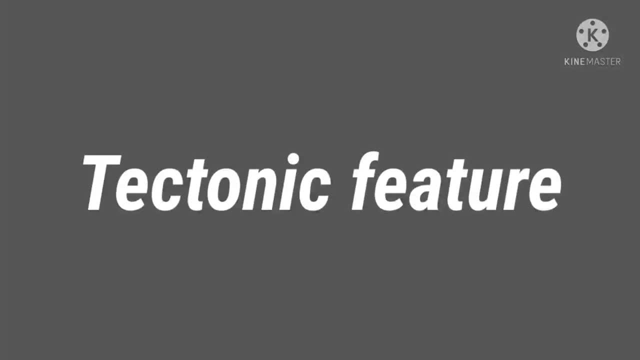 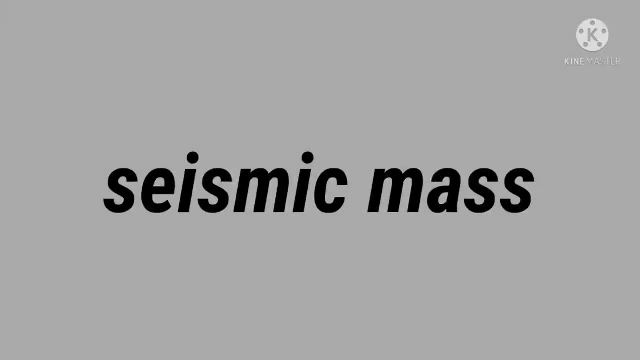 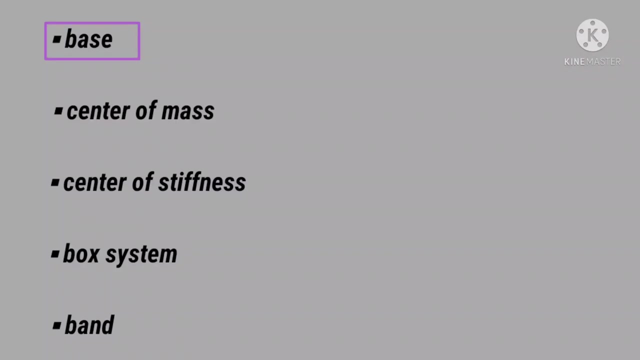 movement or quake resulting in the above consequences. Next, seismic mass. it is the seismic weight divided by acceleration due to gravity. Next is seismic weight: it is the total dead load plus appropriate amounts of specified imposed load and base. It is the level at which inertia forces generated in the structure are. 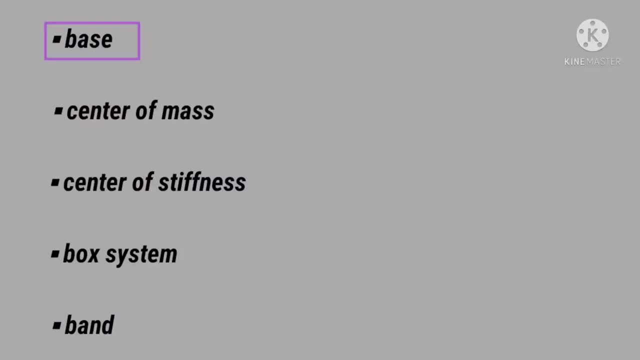 transferred to foundation, which then transfers these forces to the ground. Next is center of mass. The point through which the resultant of masses of a system acts is called center of mass了解就是 肌肉中立的重量halt, dos的體質. 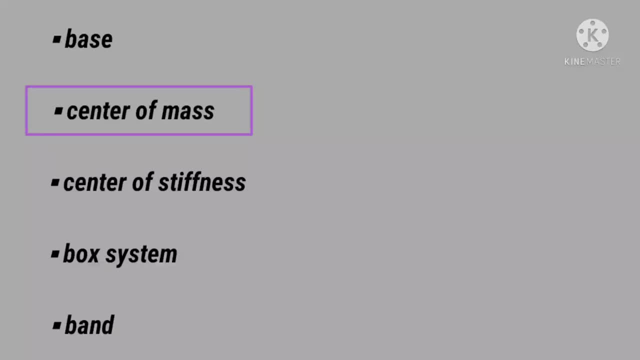 the point that means. this point corresponds to the center of gravity of masses of systems. Next is center of stiffness. The point through which resultant of the restoring forces of a system acts is the center of gravity of of mass sisters of systems. Next is center of stiffness. 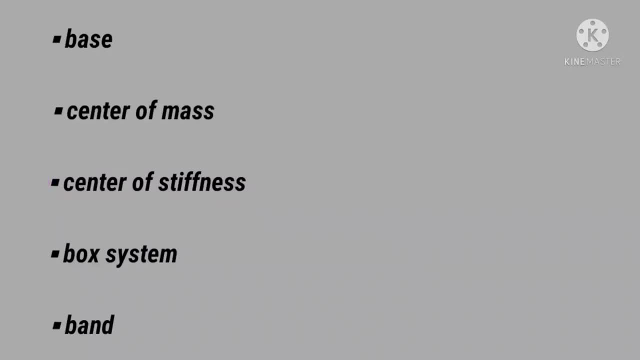 The point through which resultant of the restoring forces of a system acts is called center of stiffness. next box: system box is a bearing wall structure without a space frame where the horizontal forces are resisted by the walls acting as shear walls. band a reinforced concrete or reinforced brick. 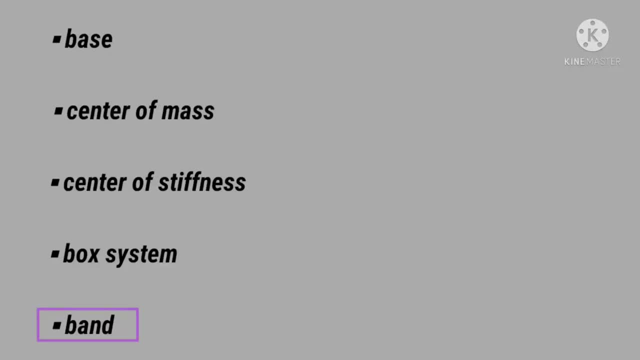 or wooden runner, provided horizontally in the walls to tie them together under to impact, horizontal bending strength in them. ductility: ductility of a structure or its members is the capacity to undergo large inner inelastic deformation without significant loss of strength or stiffness. in inelastic deformation without significant loss of strength or stiffness.